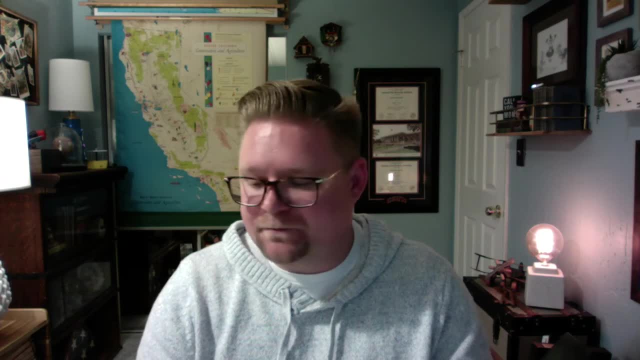 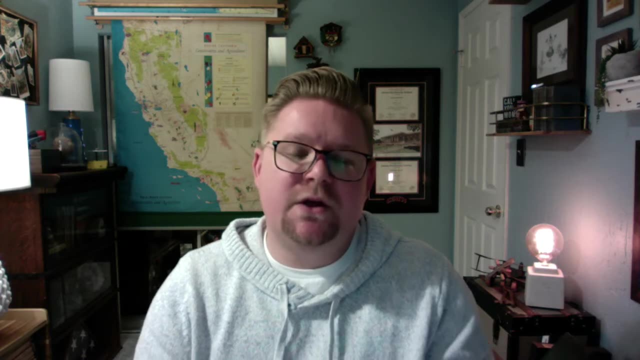 doesn't mean anything other than it's a visual category, It's a visual aspect. It'd be just kind of like, you know, anything that's orange must taste orange like an orange, And that's not the case, You know. so it's not really a valid. 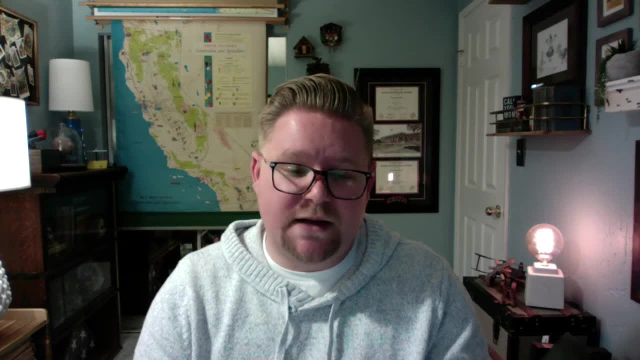 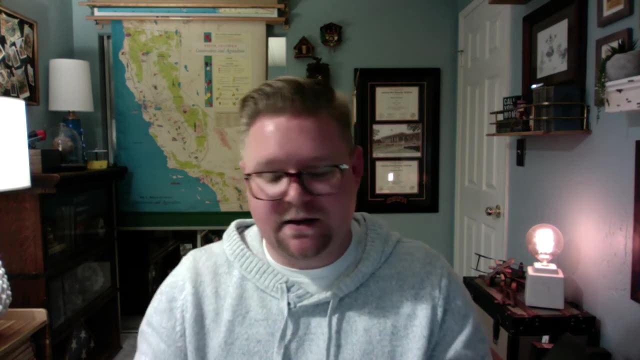 piece, especially when you try to use race to identify the way in actions and the way people act. And you know well, just because they look like this, that means they must do that, And I think that when it comes into this idea of race and ethnicity and nationality, 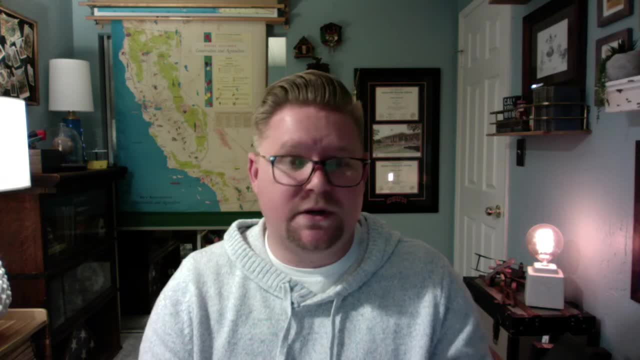 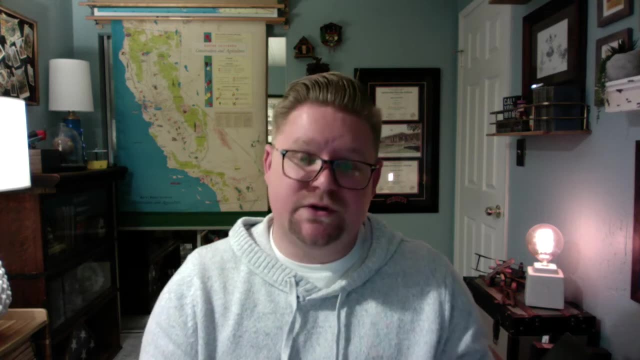 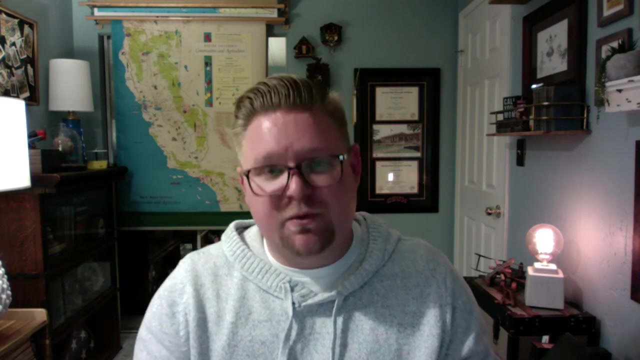 it comes in the very awkward conversation of privilege. You know talking about different types of privilege. you know there's not just- you know- ideas of white privilege, but there's also heterosexual privilege And there's also different types of ways of viewing that and to understand that certain groups have privileges. 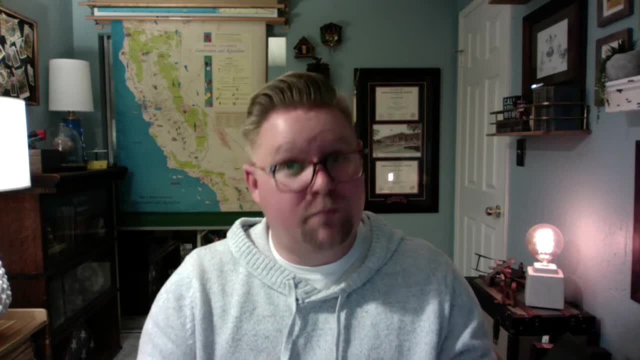 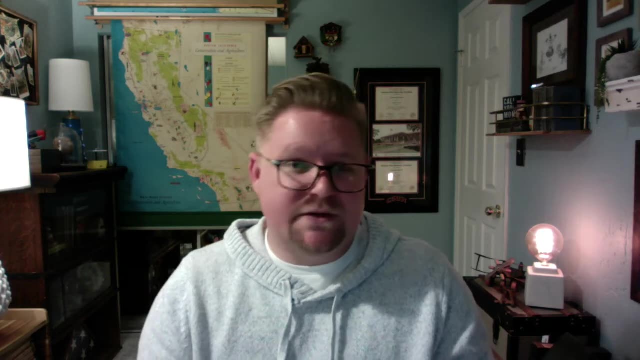 and other groups will have disadvantages. Both. everyone has a privilege. It's very different in how it's looked at, And it could be because of your gender, It could be because of your height, It could be because of your color. There's all these different attributes. 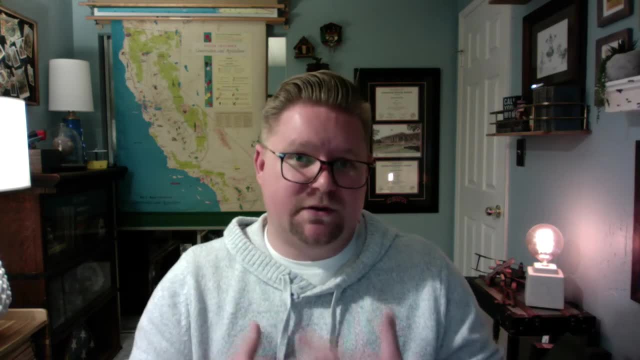 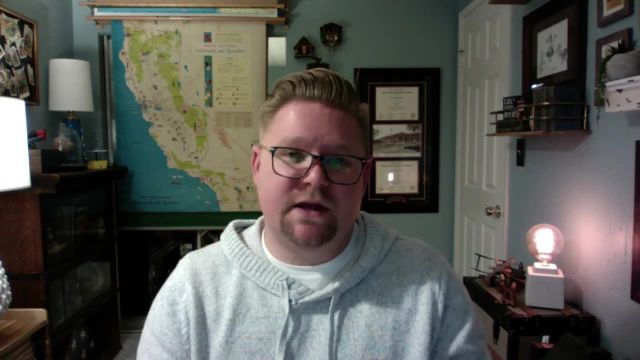 that go within that. No means am I saying that privileges are this is an appropriate way to live your life, but to understand that's the reality is that when looking at certain things that this does come through. But I think that you know what I'm saying is that you need to be able. 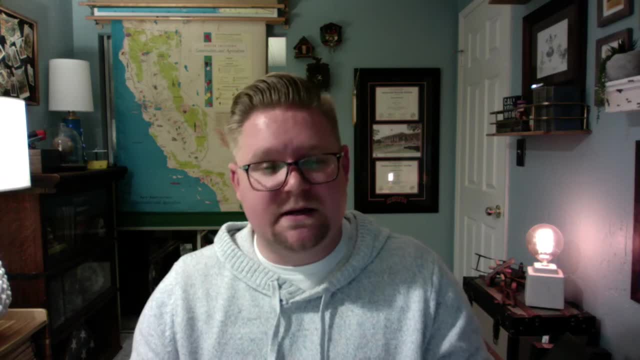 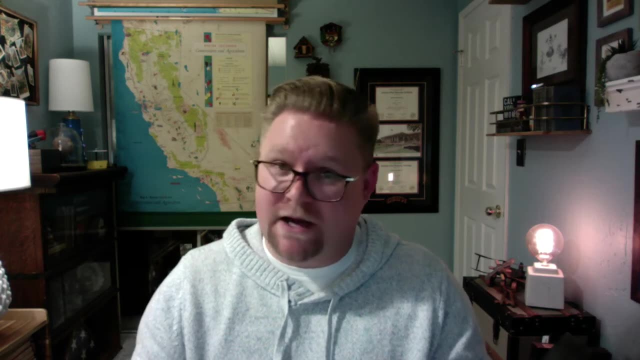 to acknowledge it and understand what that means. It's not designed to be an offensive statement That. it's not designed to be offensive to ask someone's ethnic background or cultural background. I think that's more important. I mean, you know many people, as you'll learn. 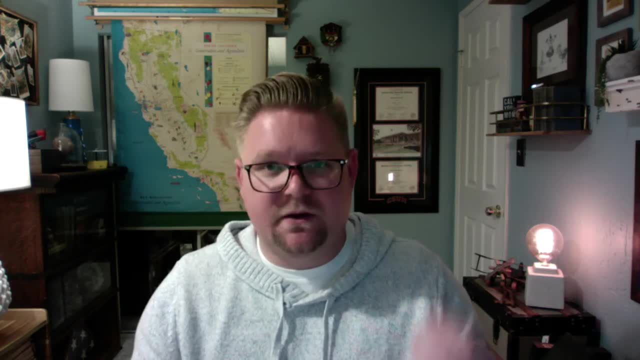 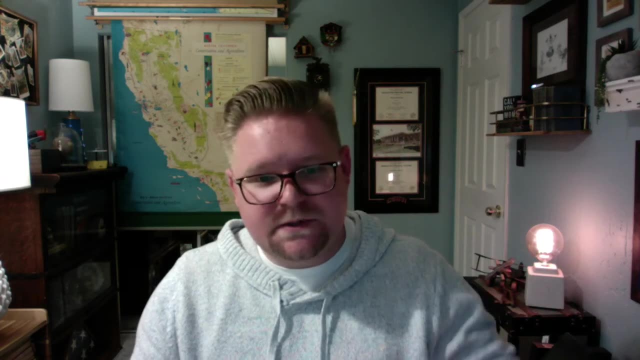 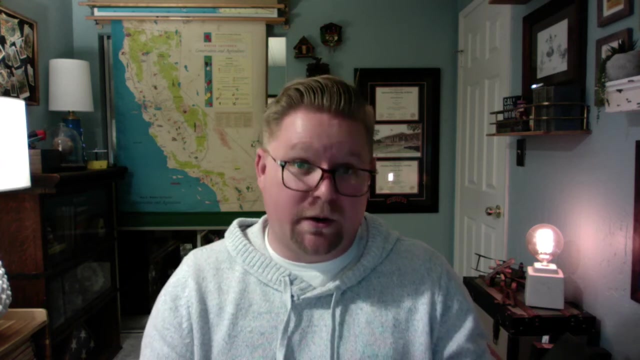 throughout this text. like people, like labels. You think people identify something or someone in a particular way, But how do we really define that? So that's what this is about: The difference between ethnicity and race- And, as you will find, the ethnic values are much more important than the racial values. 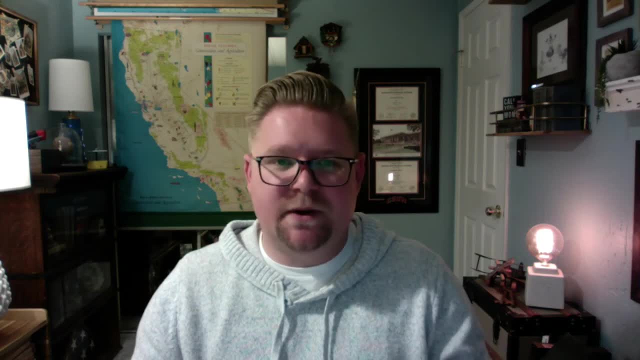 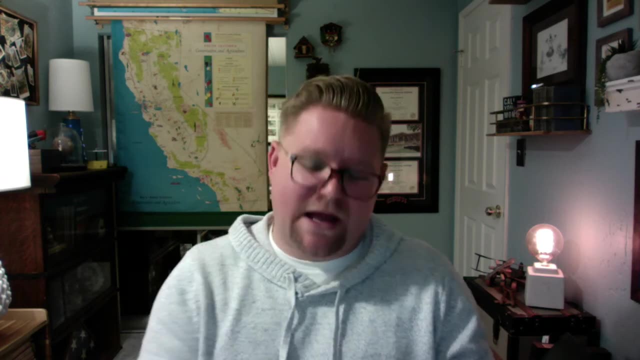 As an example, we see a lot- and the author does a great job with this- by comparing ethnic pieces to food- That we have these ethnic flavoring and spices locations- How does that reference? how do we identify that, you know? I think that's a much easier way to comprehend. 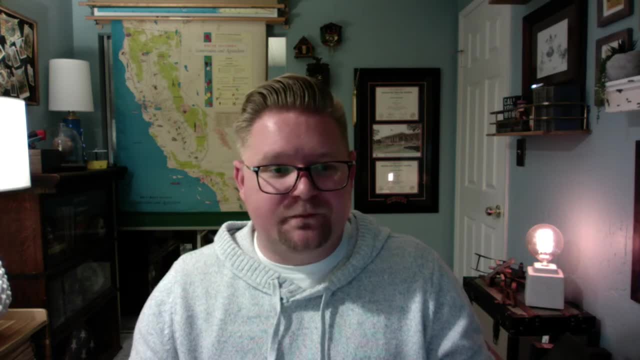 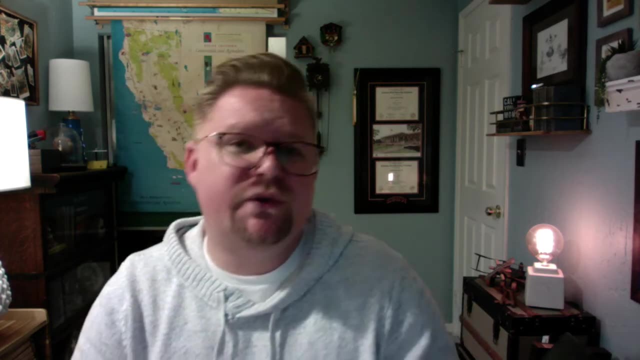 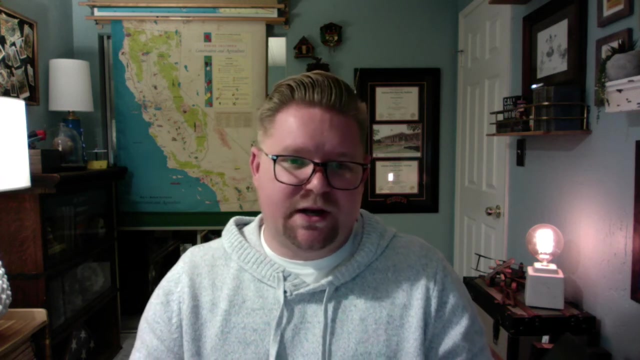 ethnicity is through food and to look at through that way, then, moving forward, we find that also ethnicity has has, you'll see, those correlations with religion. there's correlation with space and time, and so it really works out a lot easier that way. something else that the book kind of covers. that I thought was quite 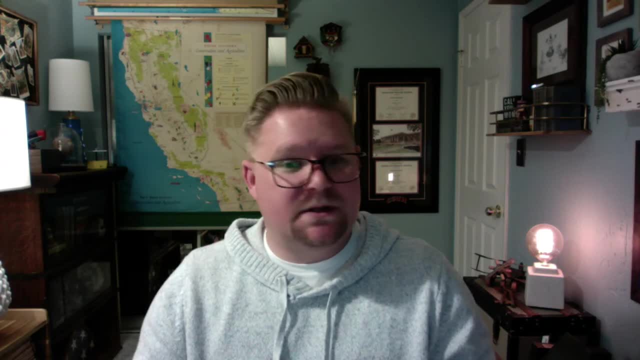 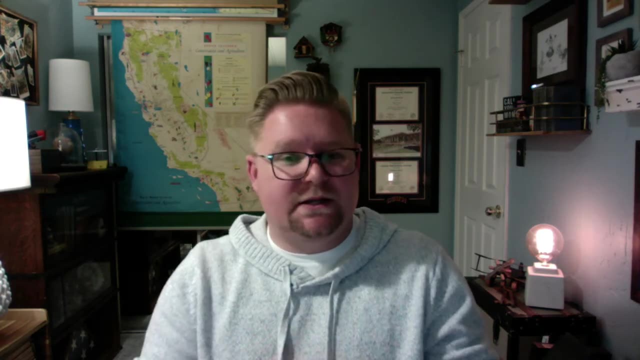 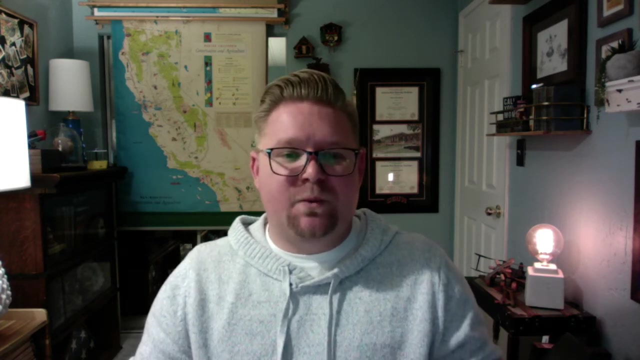 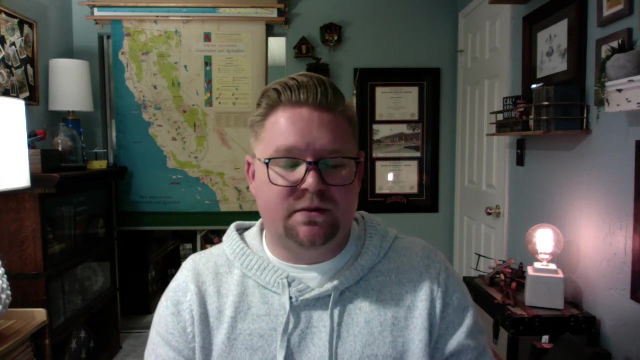 interesting is looking at, then, ethnic landscapes, not just certain areas you know by space in place, but actually looking at the landscapes, looking at the design, palm trees or adobe huts, or really what we consider in in a cultural geography. there's this term that we use: it's called the buzz and woody era, which 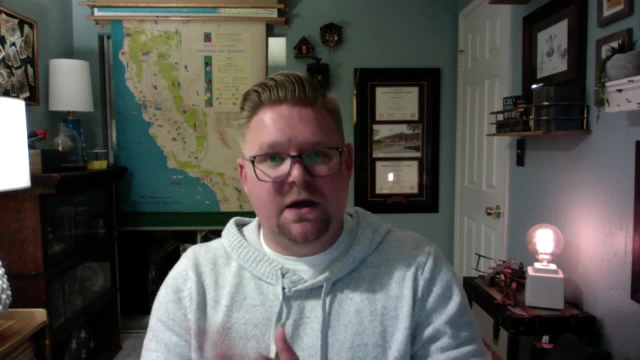 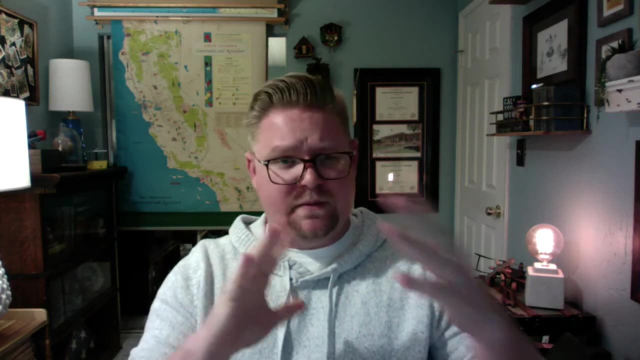 makes reference to space age being the buzz and the woody being more of the cowboy themed you know. so, looking at ethnicity themed tourism- perhaps you've seen there the hotels are made out of concrete but they look like teepees, which was a huge market in the 1950s on route 66 was. 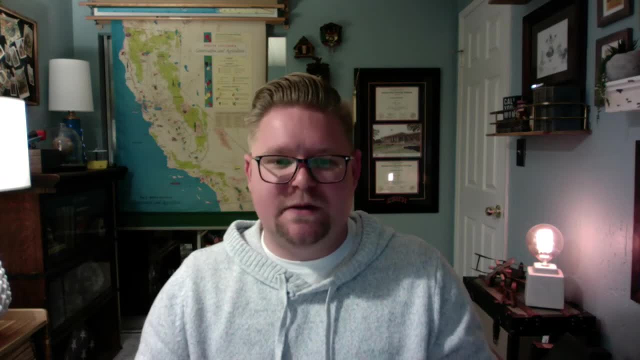 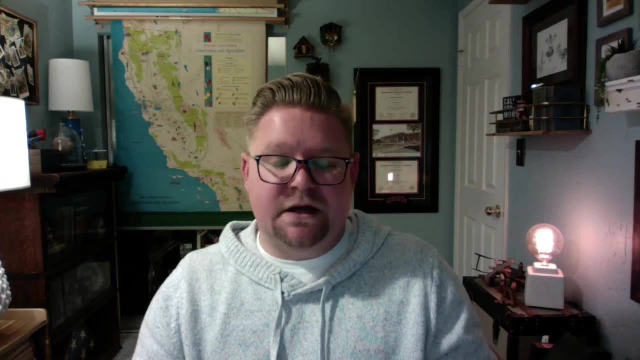 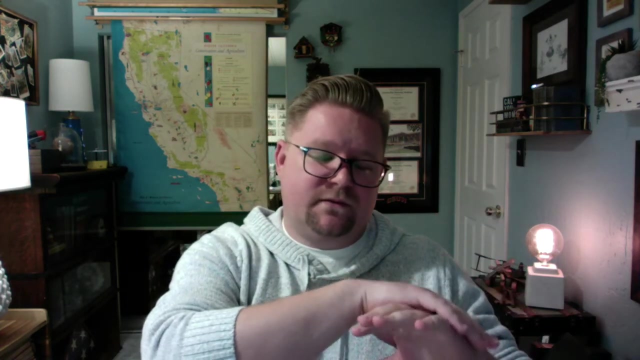 to be able to, you know, experience the American West, to be able to see these different attributes. we also see mascots, first for sports teams, you know. you can see, in particular, Sequoia National Park. their big sign used to have the face of a Native American with a headdress and that was part. so you 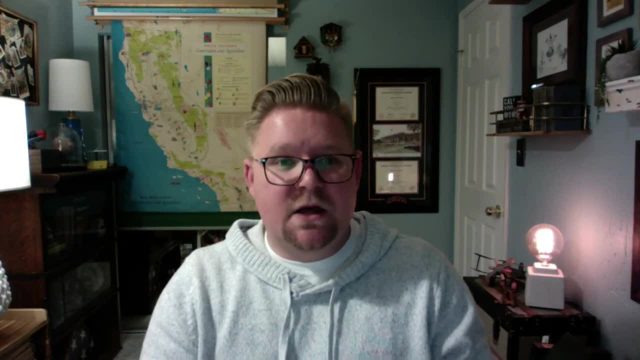 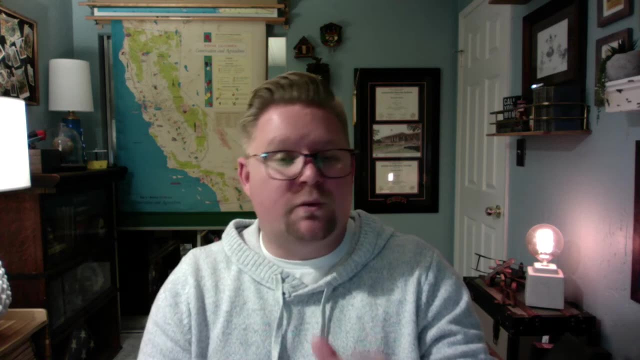 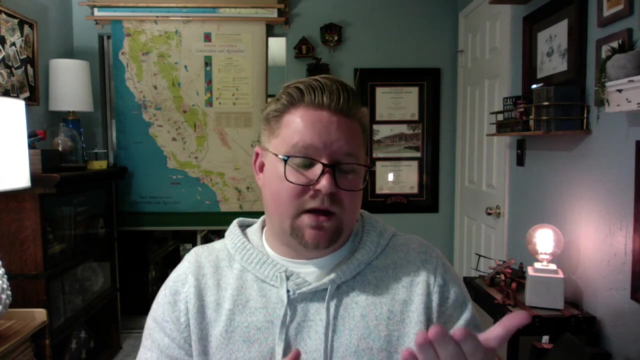 know that's where it comes into interpretation as being that are the whose benefits from this? is this designed to be racial or racist? being that, you know one is better than the other. that's what the idea of racist means. or is this perhaps culturally insensitive? it depends on the. 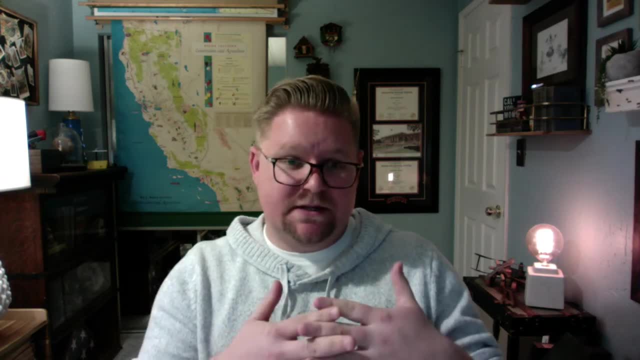 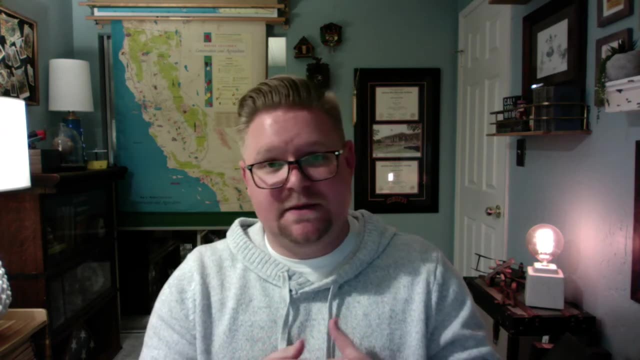 people you speak with, because in some cases some of these ideas and landscape attributes are reminiscent of of a different time. but in other cases it can be done in some form of derogatory term And the big question for us as geographers is to sit back. 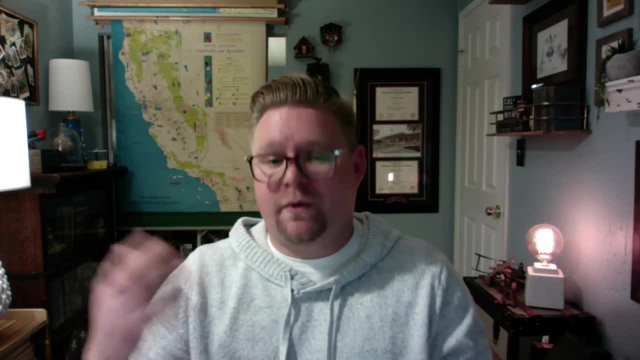 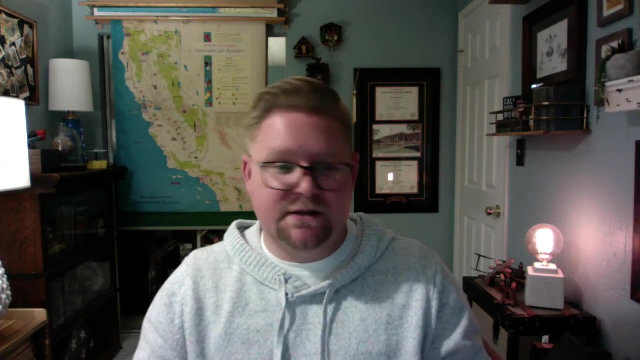 and observe it and try to understand both sides. You know, is it appropriate to have an athletic team called the Redskins? You know, and then you bring in that conversation And I think that those are things and again, I think that when we come to human and cultural geography, there's a lot of 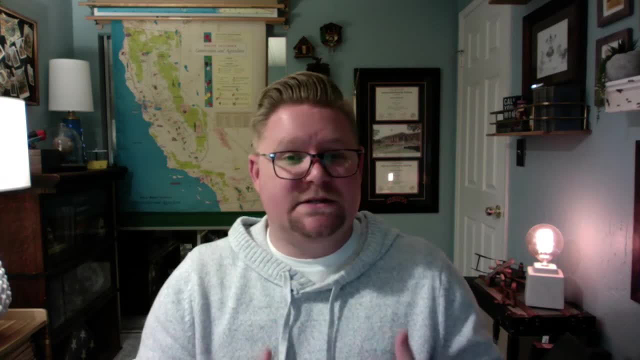 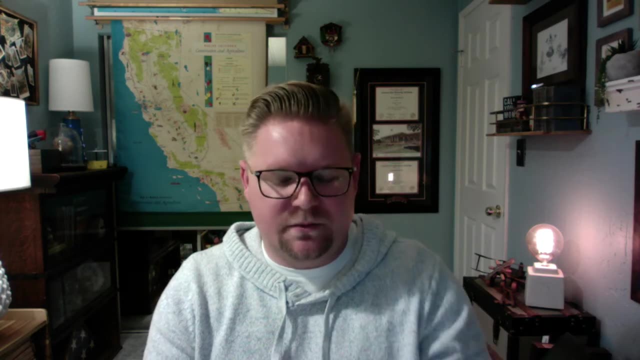 topics that become very uncomfortable, But I think it's important to bring it up because it's a way for us to listen to both sides. I heard a great conversation. It was a TED talk that I was present at, and they talked about the team, the Redskins, And they had obviously different groups of people. 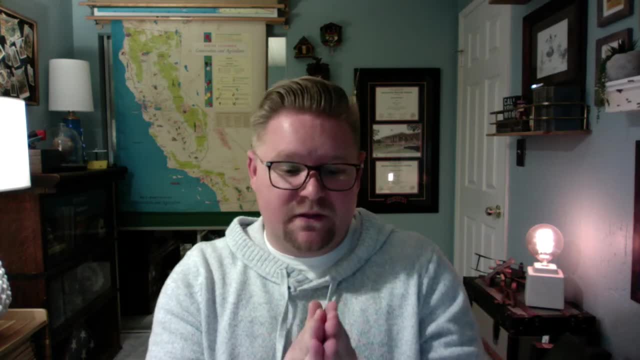 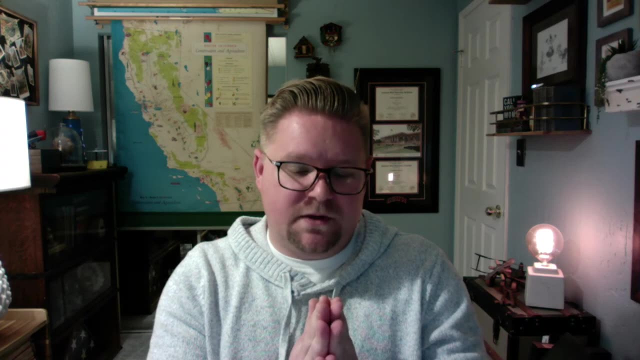 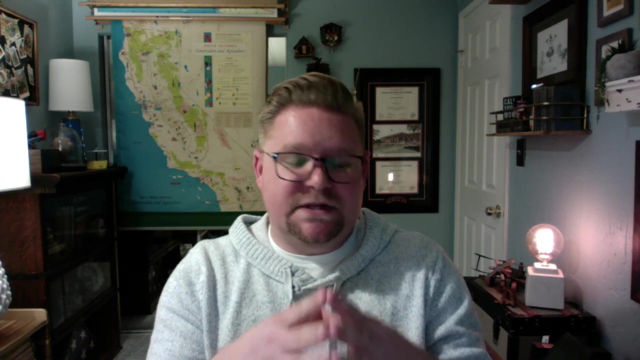 discussing, you know, the offensiveness versus the acknowledgement of a group of people you know and how some people- some of the Native individuals from where that team was found- felt that it was a way for them to signify that they were a group of people, And I think that's a great conversation. 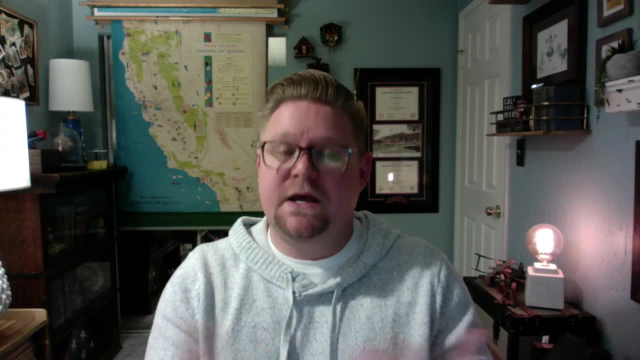 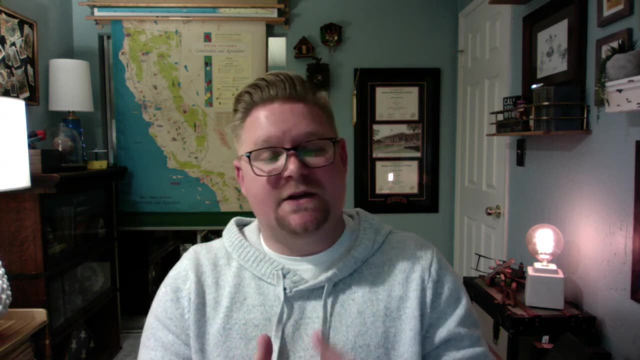 To signify and to distinguish a particular group of people to give them a prominent face in the sports world. And other people saw it as really as a derogatory statement by saying that you're going back into the idea of what are the definitions of race, and one of the biological aspects is: 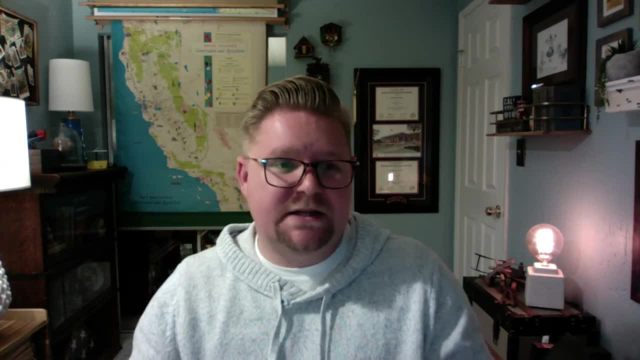 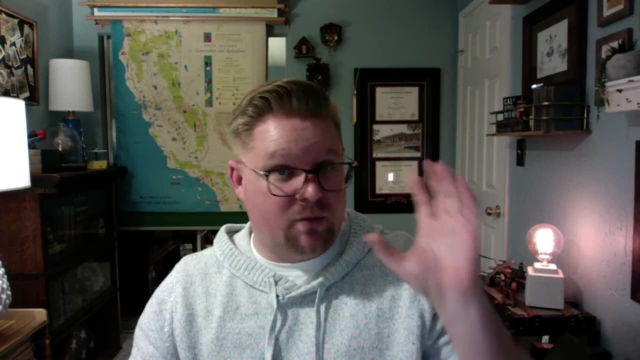 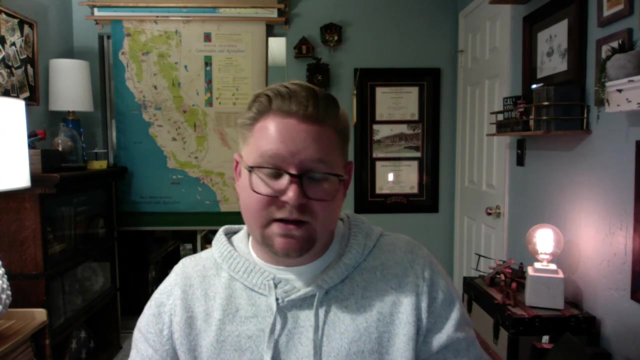 color. So, when working through this text, I think there's a lot of great ways to interpret both the ideas of nationality, which is the place that you were born, the ethnicity, which is more of your cultural influence, And then race, is more of just the visual aspect, And we'll find, and then you know, and I'm hoping, 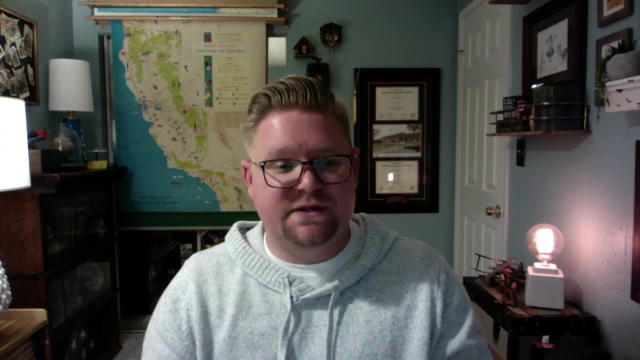 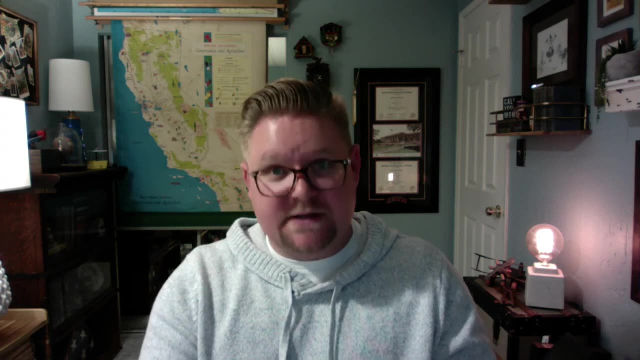 that you find that through the course of this text and through just working through this, that race is really the most useless out of all of them. You know, it's just, you know, kind of going back, especially how a lot of individuals use race to try to stereotype or try to understand. It's like 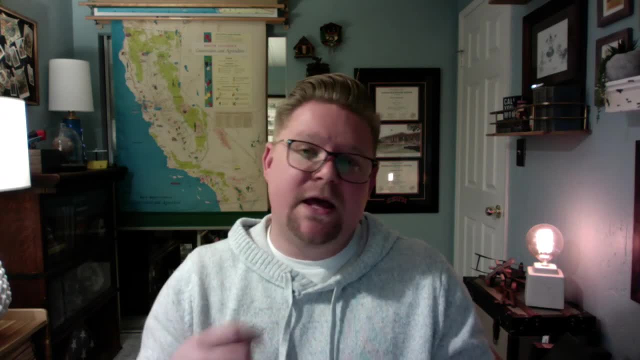 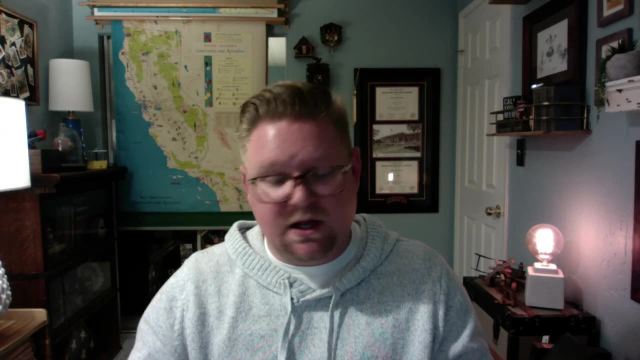 well, I ate one sour orange. therefore all oranges are sour And that's not the case. You can't, you cannot justify that statement, you know, just based off pigmentation. And we've found- that's a lot, especially when looking at crime- that there's a lot of individuals that 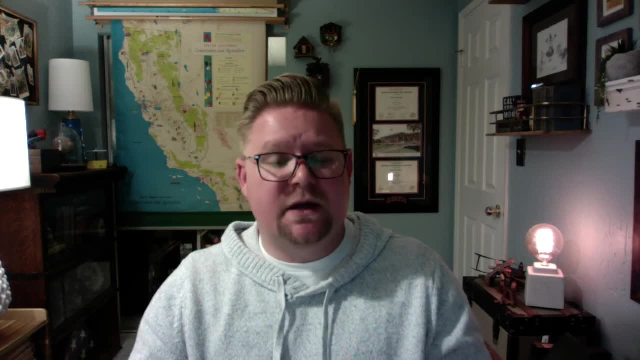 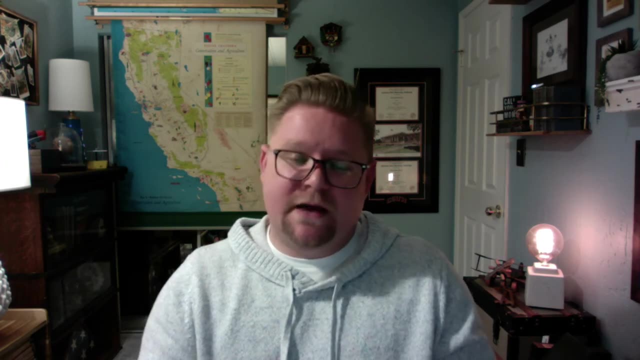 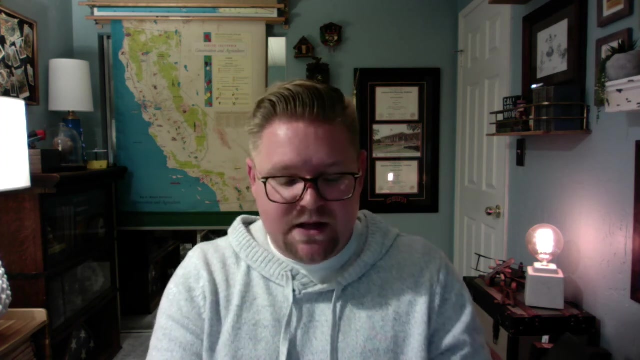 will rely on racial attributes first versus looking at some of the other elements that are at hand. And you know that's what this is really about: is to be able to understand those differences and to understand really when is a situation racist Or when is it dealing with. 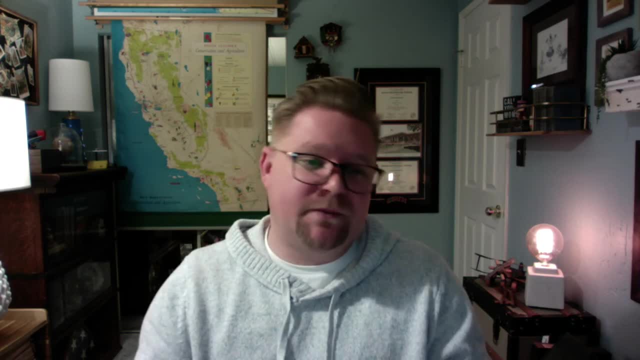 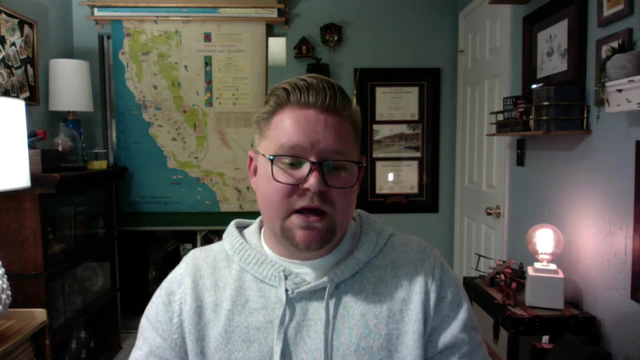 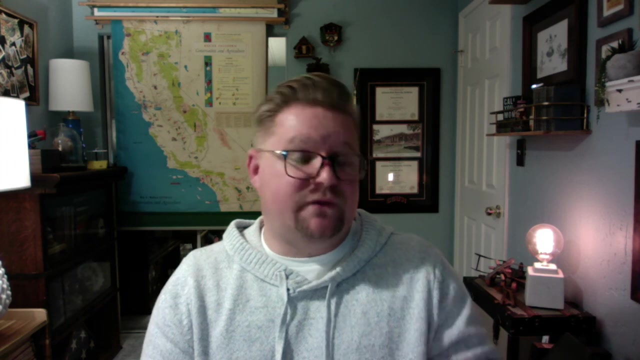 cultural insensitivity to their background. So, nonetheless, I think that you'll enjoy this. There's some great maps, some interactive aspects that discuss really the differences between, also within landscapes of what was considered white flight, And you'll learn more about that. looking at gentrification and how.